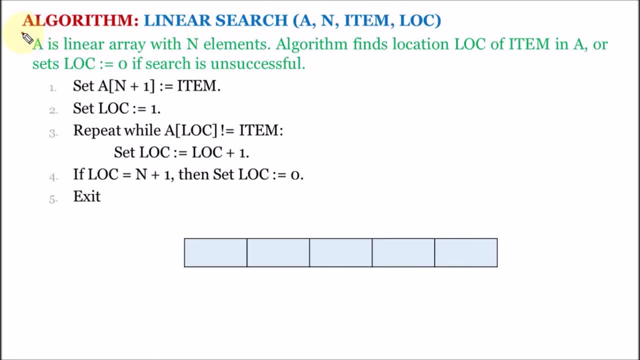 Hello everyone, my name is Ankit Verma and today we are learning the algorithm for linear search. Here we are having A- A is the linear array. So here we have taken the array whose name is A- One dimension array is also called linear array- and then we are having is N, That signify 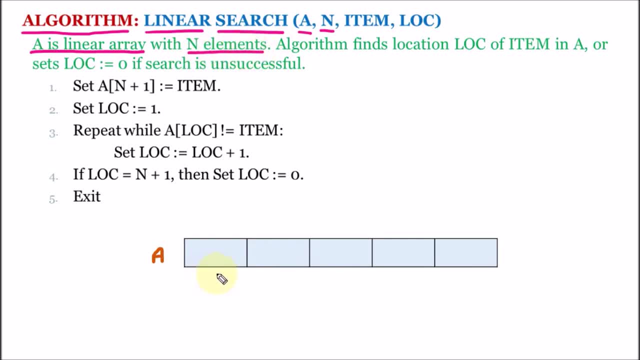 N elements. We are assuming that array contain few elements, Let's say 7, then 9,, then 11 and 13.. So these are the four elements. In the algorithm we are starting the index position from 1.. So 1,, 2,, 3 and 4.. So these are the four positions. 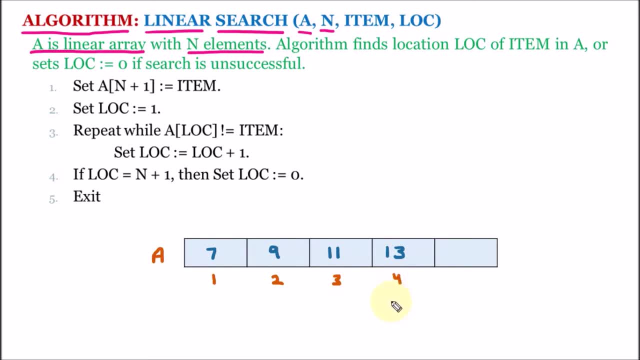 So here N signify number of elements, and we can see that here four elements are there, That is, 7,, 9,, 11 and 13.. So here the value of N is 4.. Next one we are having is item. Let us suppose we want to search 11 inside this array. 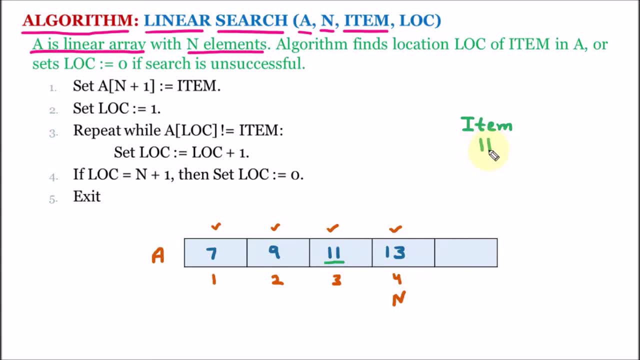 So here 11 is the item, Next one is LOC. LOC is the location of item, which is 11 that we want to search. So in that case algorithm should return the location as 3.. Here the algorithm of linear search find the location LOC of the item. 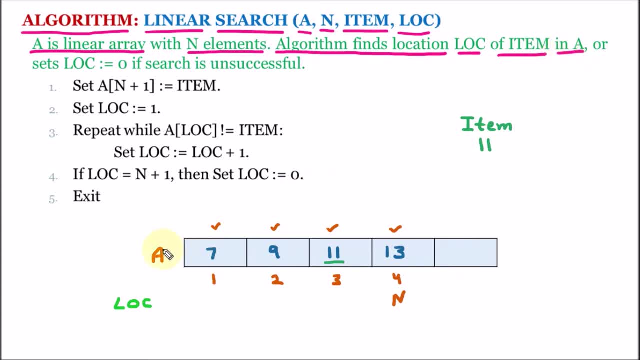 Here the item is 11 in array A, So this is the array A out of which we are finding the location, Or Set location is equal to 0 if search is unsuccessful. That means if the item not found inside the array A, In that case location will be returned as 0.. 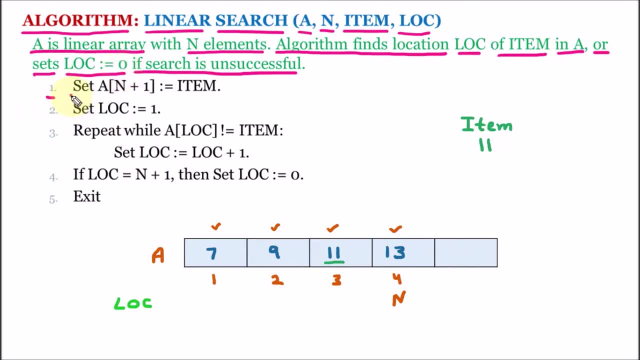 Line number one of the algorithm says: set A, N plus 1.. Here we know that A is the array and the value of N is 4 and N plus 1 means 5.. So here A5 means we are talking about this place, and that is equal to item. 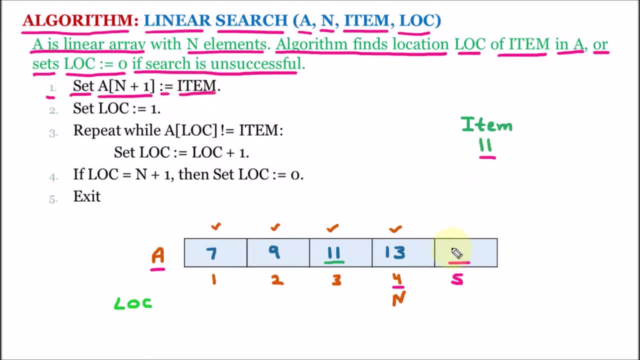 And we know that item is 11.. So we are putting the 11 on the last of array, So we are making it as the end point for the loop. So loop will break here, Then afterward in line number two. set location is equal to 1.. 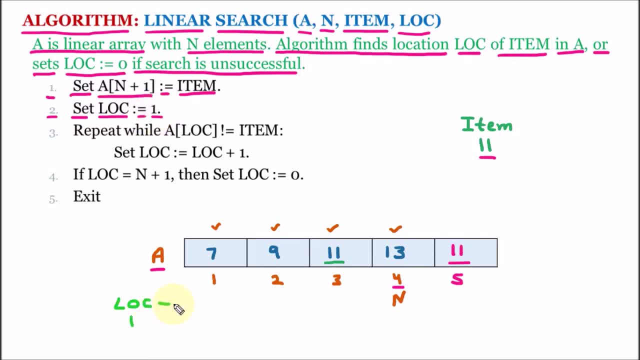 So here the value of location is equal to 1.. location is one, so that means it is on the first position in line number three of algorithm. we are saying repeat while a look, we know that the value of location is one, so here a one that means it is. 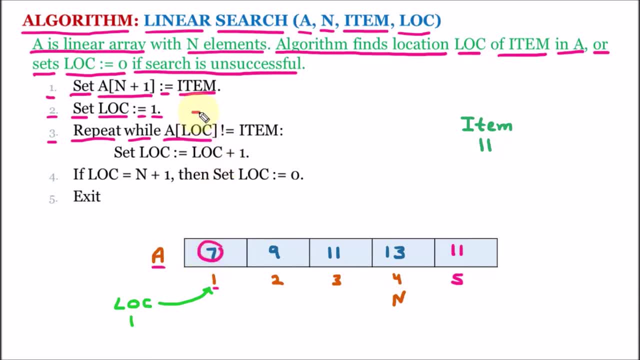 seven. so we are checking that seven that is not equal to, and we know that item we want to search is 11. so seven not equal to 11, that is true. so we are going to repeat the inner portion that is, set location is equal to location plus one. so here the value of location is incremented from one to. 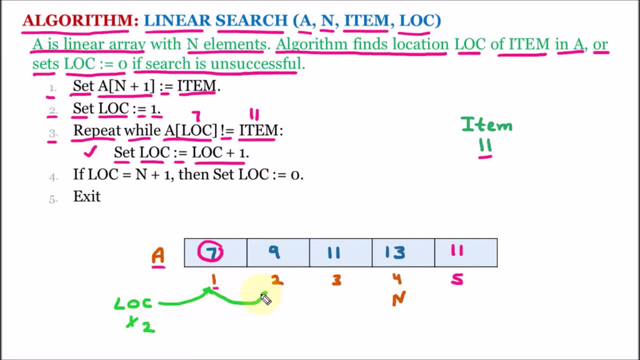 two. that means location is shifted to the next position. it is a loop, so it will be going back and again checking the condition that a location- and we know that a is the array and location is two, so a two means nine. so here we are talking about nine- nine not equal to item and item is still 11. nine not equal to 11. the condition is: 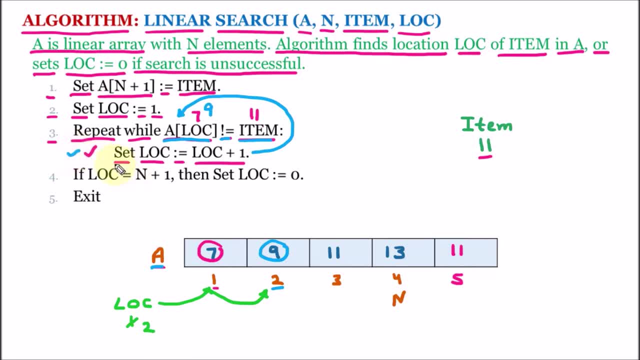 true, that means inner part will work and set location is equal to location plus one. so here the location is incremented to three and it is going to the next position. it is a loop, so again it will be going back and checking the condition and the condition is a look. we know that a is the array and the location is three. that means 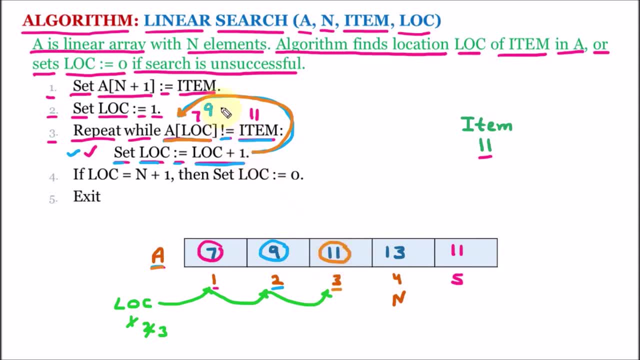 a3 is 11. so here we are checking that: 11 not equal to item and the item is still 11. 11 not equal to 11. here the condition is false because both are equal, so inner part will not work. in line number four we: